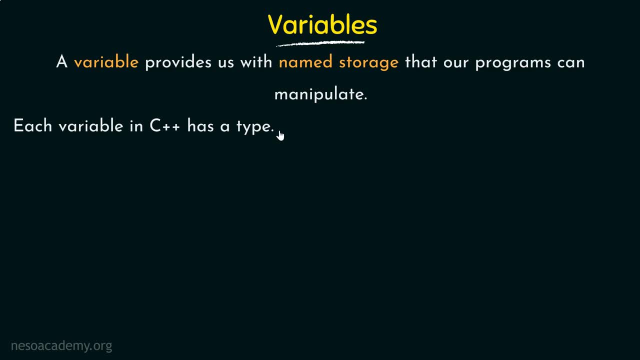 do with integers. So the type will tell us many things like what we can do with that variable and what are the kind of operations that can be performed, etc. So let's see a little more in detail about that. So, as we said, type determines the size and layout of the variable's memory. So first of 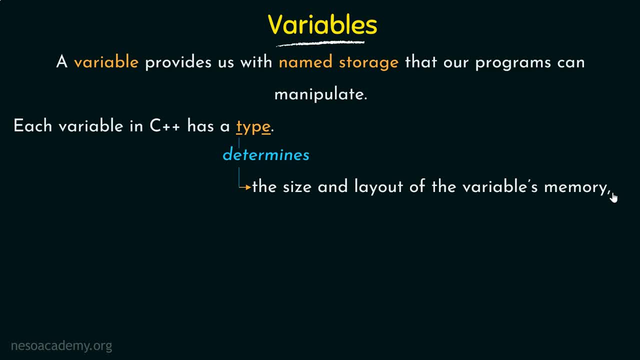 all the type will tell us the size and the layout of the variable's memory. So in one of the previous lectures, when we discuss about the various types, we have already seen the amount of memory that is occupied by different types. So we have seen, like, how much memory is occupied by integers, how much. 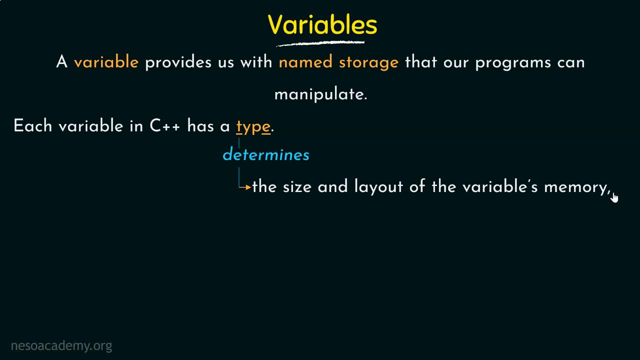 memory is occupied by characters and so on. So the type will tell us the size and the layout of the variable's memory and also it will tell the range of values that can be stored within that memory. So this also, we have already seen the range that can be stored. So when we say integer, integer has 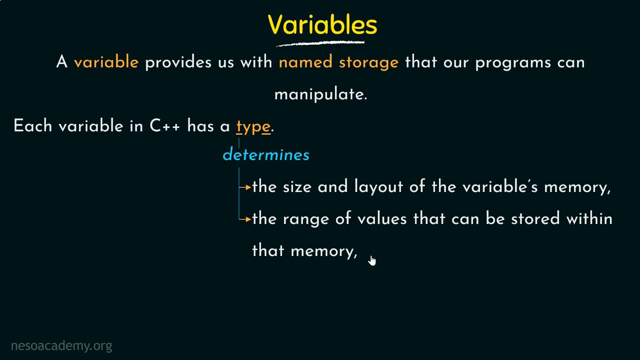 the same value as the number of numbers that can be stored within it. Now if you want to store bigger values, we'll need to use other types which can store larger range of values. So type will also tell us the range of values that can be stored within that memory and also the set of operations. 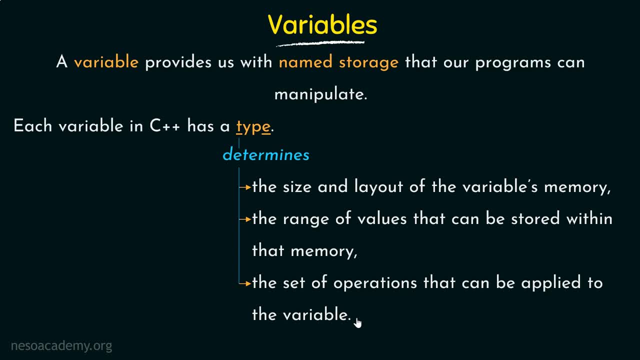 that can be applied to the variable. So it will also tell us the kind of operations that can be performed on that variable. So, for example, if we have an integer, we know what are the basic operations that can be performed on integers. And suppose we have characters. 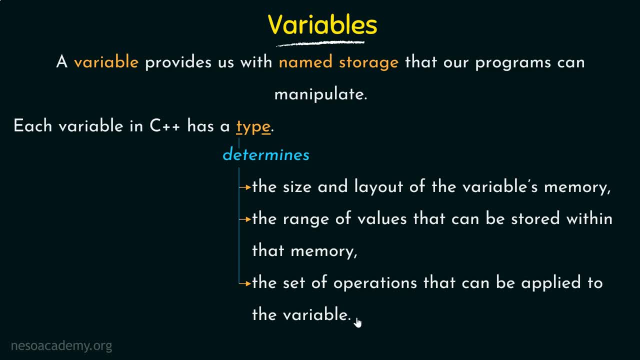 We know the type of operations that can be performed on characters. So the type of operations that we perform on integers and characters will not be the same. So the type also determines the set of operations that can be applied to the variable. So we have seen that. 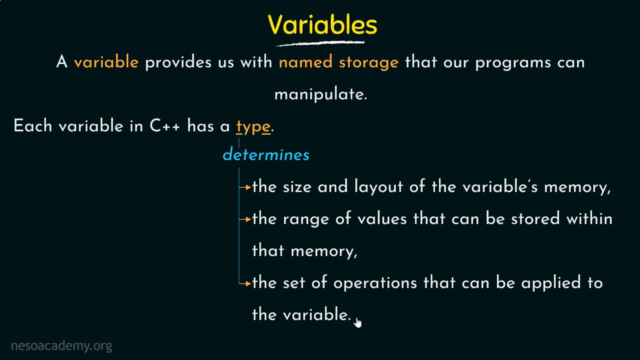 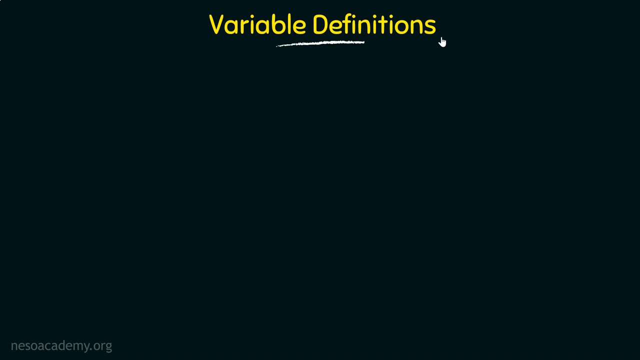 variables are a named storage, and then also, they have a type associated with them which determines these things that we have seen in this slide. Okay, now. next, let's see how variables are defined. Now coming to variable definitions, how variable definitions are defined. So let's see how are variables defined in C++? So by. 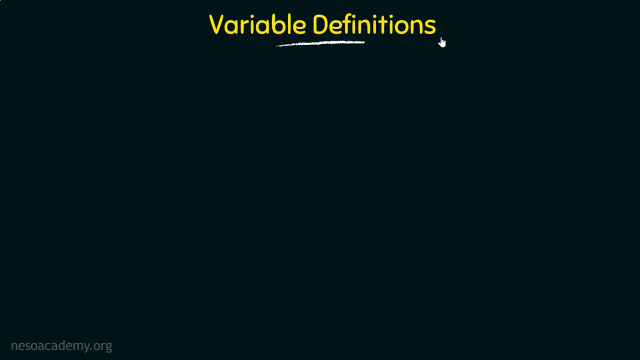 variable definitions. we mean, whenever we are trying to make use of a variable, how are we going to make the compiler know that we want to use that particular variable? And then, how are we going to make the compiler know what type of variable it is and what are the values that it needs to take? 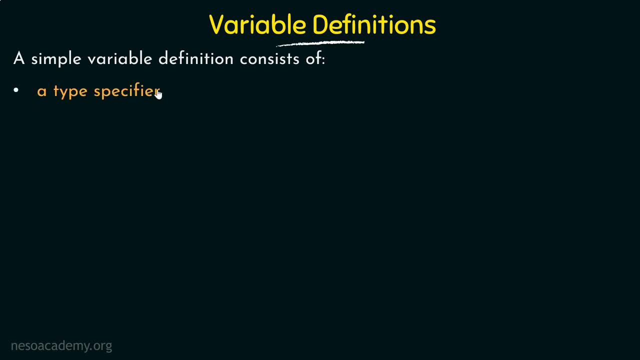 So a simple variable definition consists of the following things. Let's see so. first of all, it has a TypeSpecifier, So TypeSpecifier is nothing but the type. a So int. a So int is the type, So int or integer is a type. So that is a type specifier. 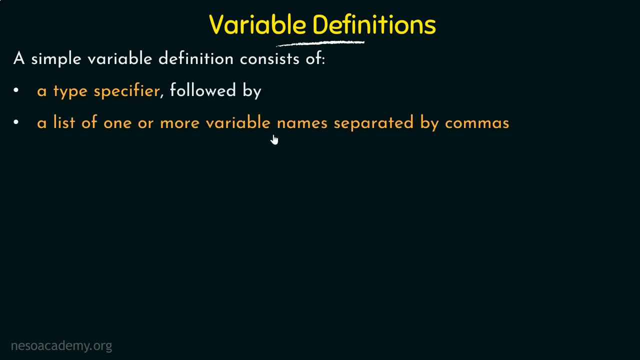 that we are talking about. Then next a list of one or more variable names, separated by commas. So the type specifier that we have discussed will be followed by the variable name. So suppose we are just declaring or defining just one variable? then we are going to just put one. 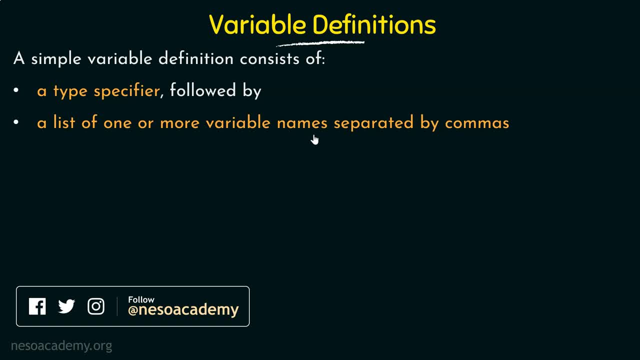 name, For example int a. Now if you want to declare more variables of the same type, then you can separate them by commas and you can declare more variables of the same type. So we will see examples to make it clearer. And then it ends with a semicolon And we have to end the 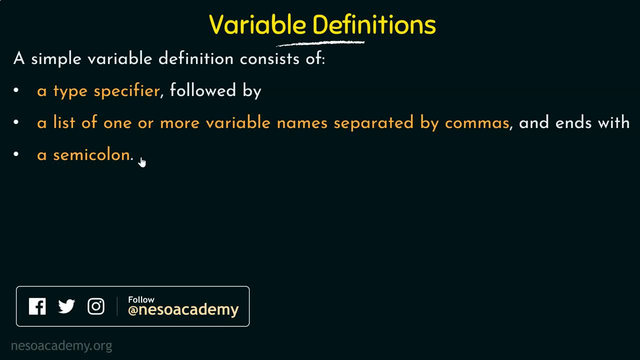 variable definition with a semicolon, like all the other things that we end in C++ statements. Okay, So let us see some examples. So, for example, here we see, here I am declaring a variable named no num1, and then it is of the type integer. So this variable definition consists of the type: 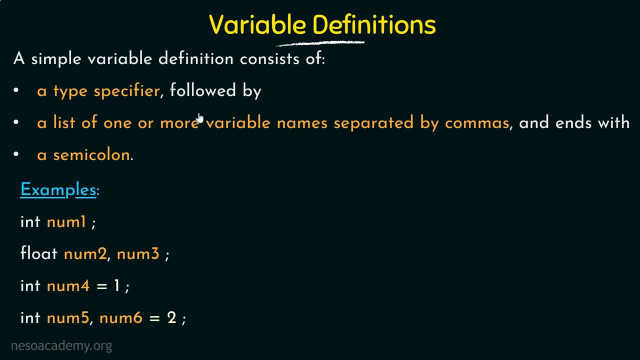 specifier, that is int, that is an integer, and followed by the variable name. So what is the variable name? num1.. This is a variable name and it ends with the semicolon. So we see it ends with the semicolon. So this is how we can define the variables. So here in the second example, 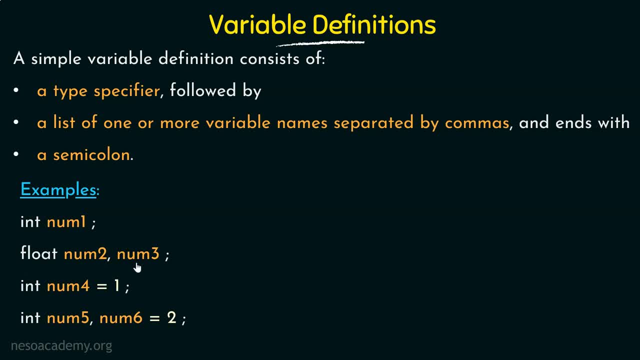 we have float num2, num3.. So what does this mean? So this means that I am declaring a variable of the type float, which is num2, and I am declaring another variable, num3, which is of the same type that is float. So we see float num2, num3.. So this comma tells us that we are declaring: 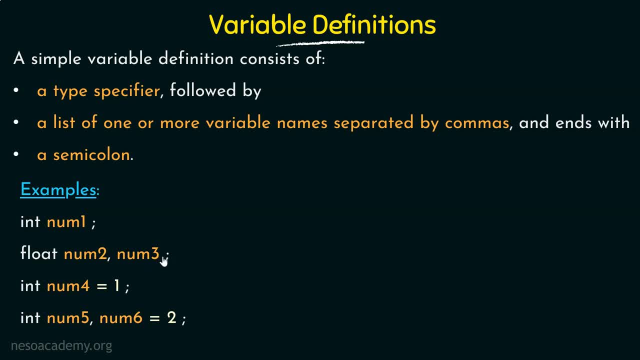 one more variable of the same type that is float. So you can give commas and keep on defining more variables, but they will be all of the same type. that is float and it ends with a semicolon. So this is another way of defining variables. 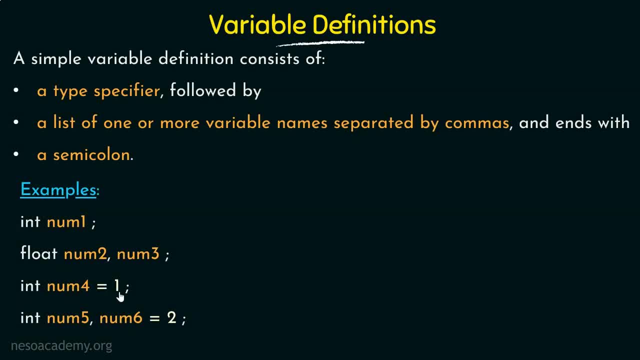 So what does it mean? here It looks a little different from the other two examples that we have seen. So here it is nothing. but we are trying to declare a variable of the name num4 and then of the type integer, and then we are initializing the value to 1.. That means while 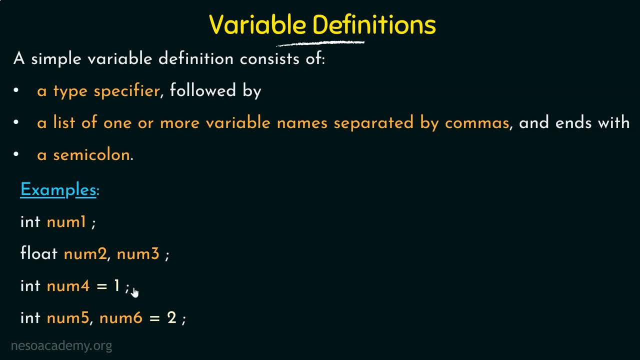 declaring this variable itself, we are trying to give an initial value to this variable called num4.. So in the previous two examples where we declared the variables integer num1 and float num2 and num3, we did not give any initial values. So when we don't give any, 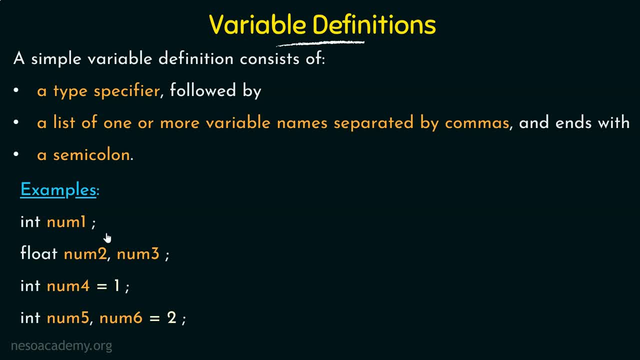 initial values. C++ will assign some initial default values to these variables, But we also have the power and feature in C++ to initialize the value at the time of declaration itself. So like, for example, here we are declaring a variable of the type integer, of the name num4. 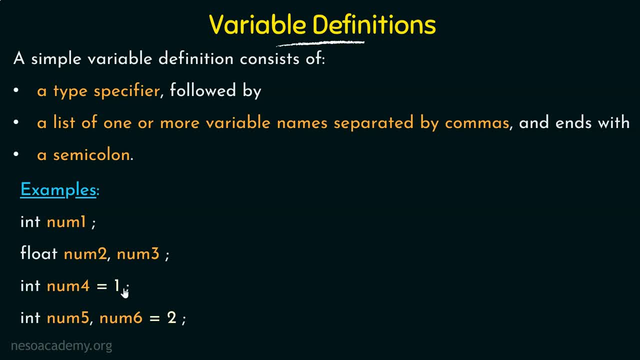 and we give the value equal to 1 here itself and it ends with a semicolon. So num4. will have the value 1 and it is of the type integer. Now, similarly, here I am declaring two more variables, num5 and num6.. So num5 of the type integer, and then I give comma here. So 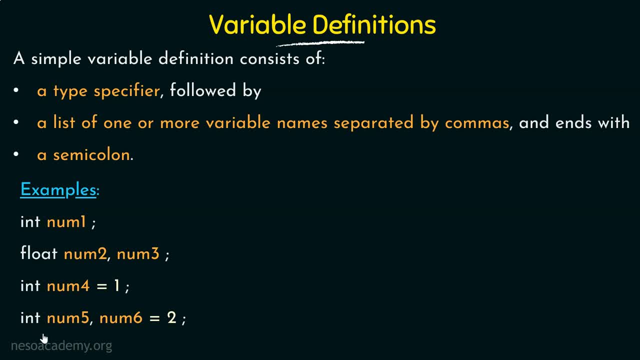 when I give comma, what happens? int is going to be continued. That means the next variable that I declare also is going to be of the type int. So I declare one more variable, num6, and then I am initializing only the value of num6 to 2.. So num6 will hold the value 2 and then num5. 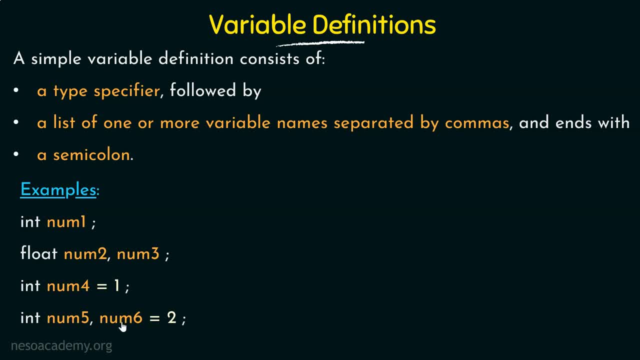 will have some other default values. So these two things that we see here, they are known as initialization, So we are initializing the values at the time of defining the variables itself. So that is one feature that we have in C++. Okay, so let us try to run this program. That means: 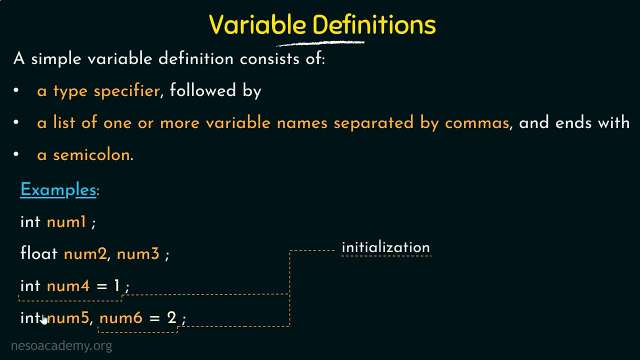 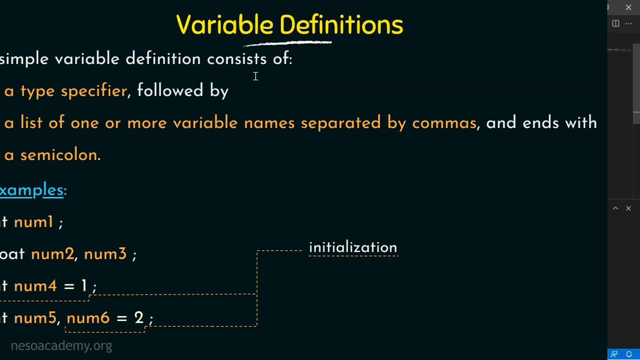 let us try to just declare these variables or define these variables like we have shown here, and then let us try to just print out the values and see how does it work. So here I come to Visual Studio Code, and then here this is the part that we have seen in our 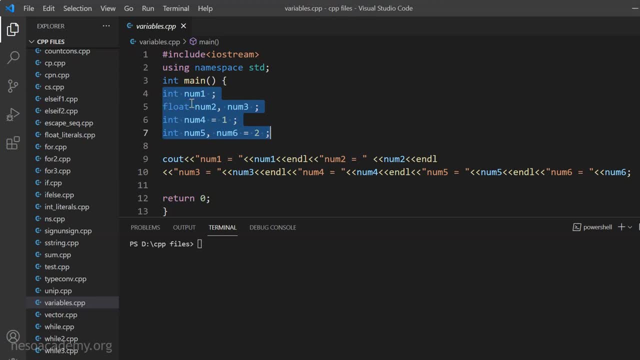 slide, So I am just writing the complete program. So here I have declared int num1, then float num2 and num3, then int num4 equal to 1, then int num5 and num6 equal to 2.. Now 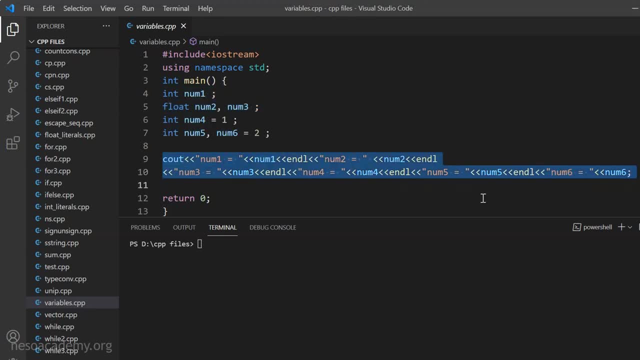 here I am trying to print out the values on the screen. So what am I doing? I am just using the seeout statement. Then I am saying num1 equal to, and then the value of num1.. Then nline- that means I am going to a new line. Then num2 equal to value of num2, and then again. 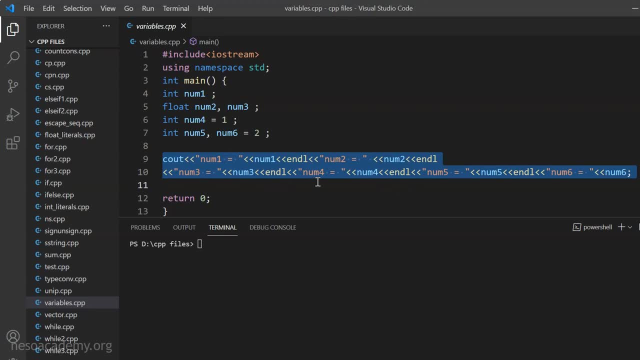 nline, that means we go to a new line, and similarly for num3, num4, num5 and num6.. So basically it is nothing, but it is just going to print the values all in new lines. So let us see. 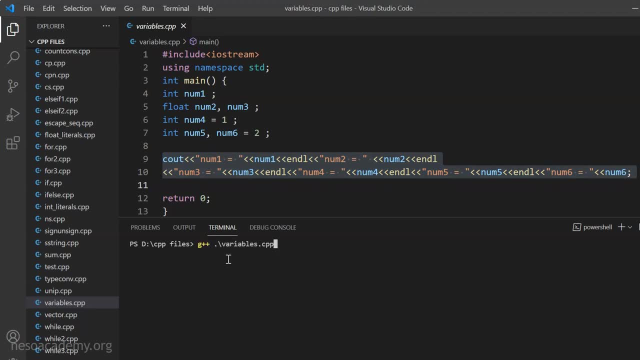 how they work. So let me compile this program. So the name of the program is variablescpp. So we type g++, variablescpp and I press enter and we see the program got compiled successfully. There is no value, 0 or 0. Now let me run it. Okay, slow, dot slash, a dot exe, which is the name of the. 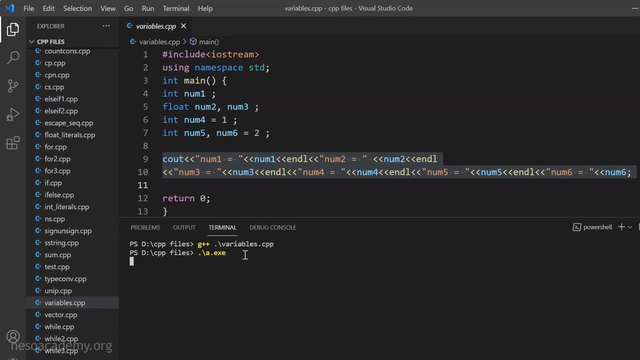 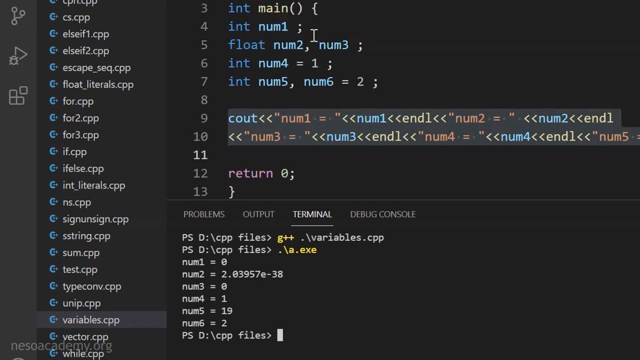 output file that got generated. I press enter again. Let us see what is the output. So here we see int num1.. We just declared int num1, but we did not give any initial value. So c++ just gave the value 0 to it. So the default value 0 is assigned to it. Okay, now what about this one? 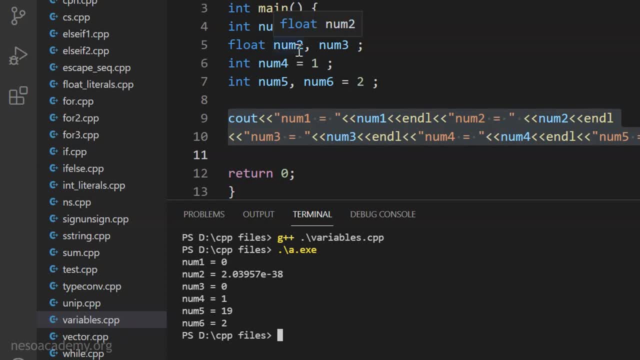 float num2 and num3.. So in case of num2, we see there is this value 0 and num3.. So in case of num2, we see there is this value 0.. So we are going to print this output file. Now, what about this? 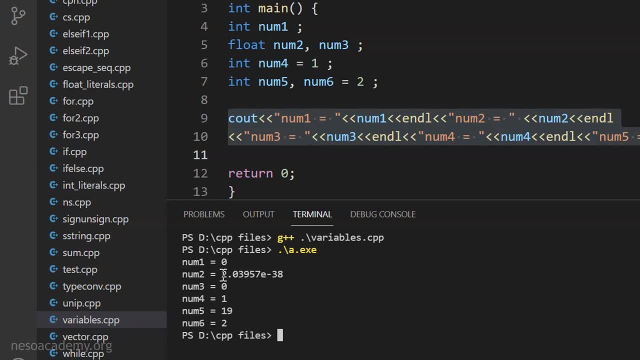 we see there is this value that is printed. So some decimal value is printed here, which is some default value which is given by the compiler itself, and then num3 is given the value 0. So we see, when we are not initializing it, C++ just gives some default random values to it, and then num4. 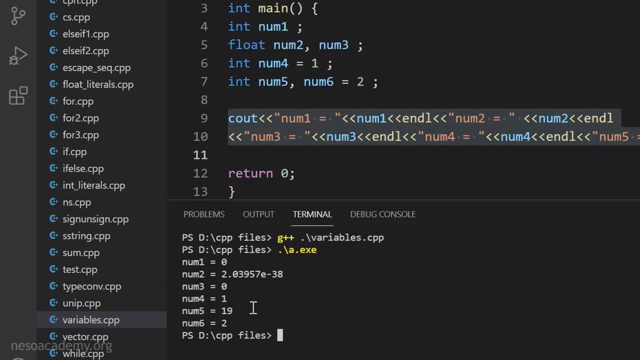 equal to 1.. So since we already initialized the value of num4, it is having the value 1.. So since we said we want num4 to be equal to 1, so num4 is equal to 1 and again here we declared num5. 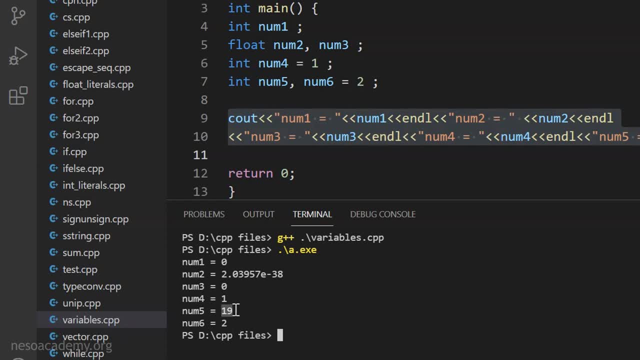 but we did not initialize it, So it gave a default value, 19, to it, and then num6 is equal to 2.. So we already initialized the value of num6.. So num6 is equal to 2.. So we see that whenever we declare a 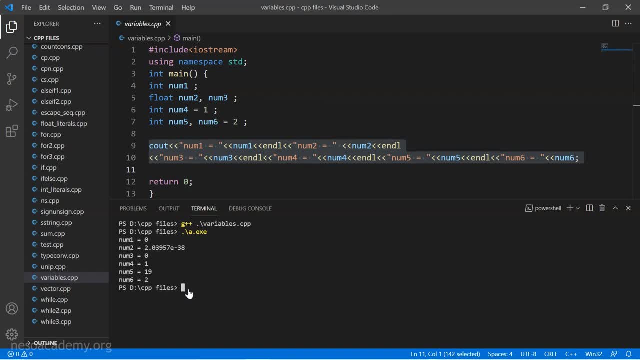 value without initializing it. C++ is just giving some random default values to these variables. So we have to be very careful when we make use of variables such as num4 and num5.. So we have to be very careful when we make use of variables such as. 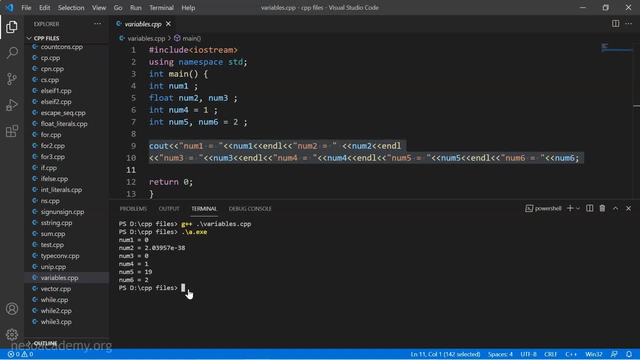 that are not initialized. So sometimes when you are doing some calculations and if you are going to make use of a variable that has not been initialized and you did not even assign any values to it in the course of your program, So making use of those variables in your calculation,